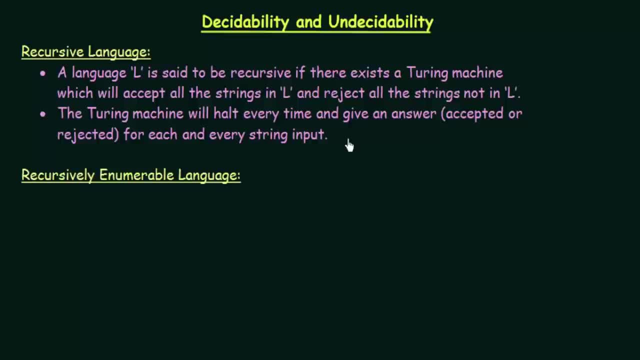 the Turing machine for recursive languages will always hold. That means the Turing machine will not go into a loop, So it will either accept the language or it will reject the language. If the string is in the language, then the Turing machine will accept it. 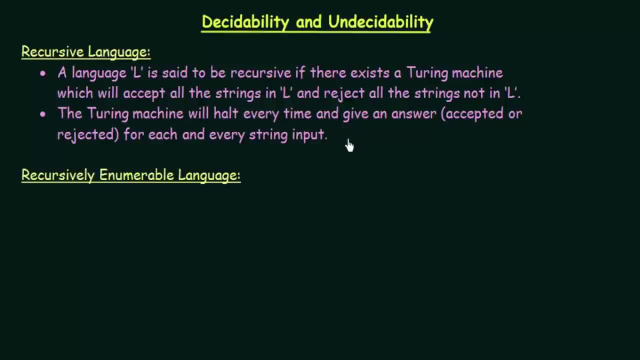 and if the string is not in the language, the Turing machine will reject it. So that is recursive languages. Now let us see what is recursively enumerable languages. So a language, L, is said to be a recursively enumerable language if there exists a Turing machine. 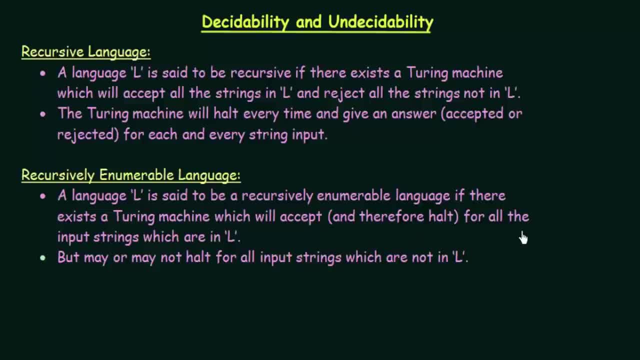 which will accept and therefore hold for all the input strings which are in L, But it may or may not hold for all inputs which are not in L, So in recursively enumerable languages. if you pass a string from this recursively enumerable language into a Turing machine, then 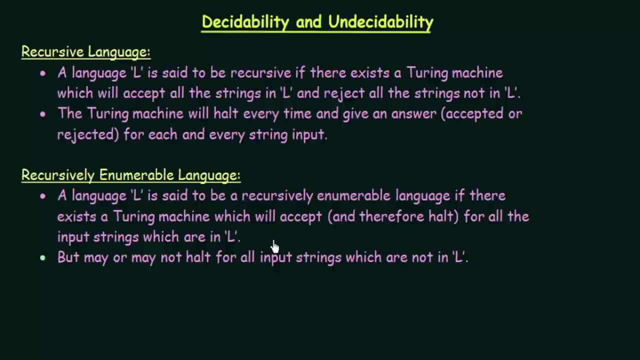 if that string belongs to the language, then the Turing machine will accept and it will hold. But if you pass a string which is not in this language, then the Turing machine may or may not hold. We cannot guarantee that It may not hold. also, sometimes 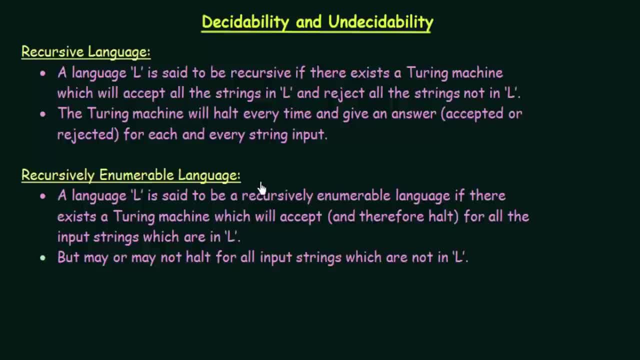 So the difference between recursive language and recursively enumerable language is that in recursive language the Turing machine will always hold. It will either accept and hold or reject and hold. But in case of recursively enumerable language, the Turing machine will hold only when. 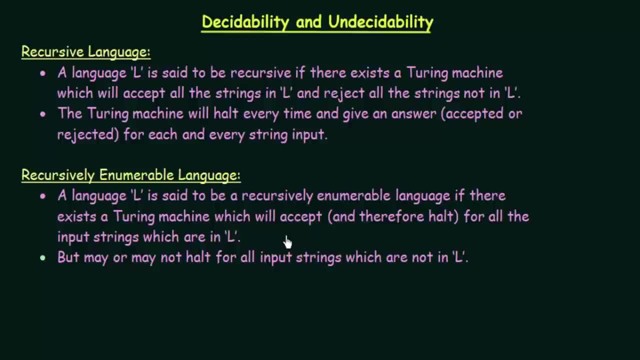 it is accepting the string in the language. In other cases it may not hold. So that is what we mean by these two sets of languages. Now let us see, by understanding these two languages, how can we define decidable languages? and partially: 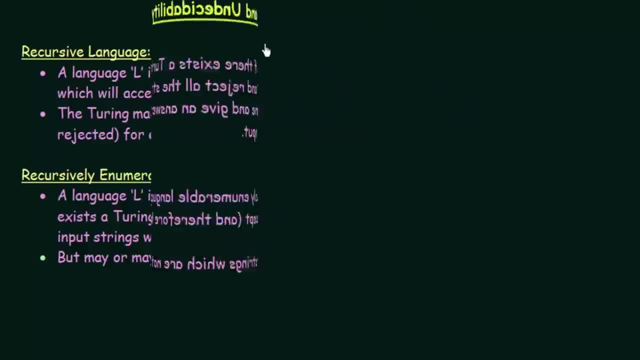 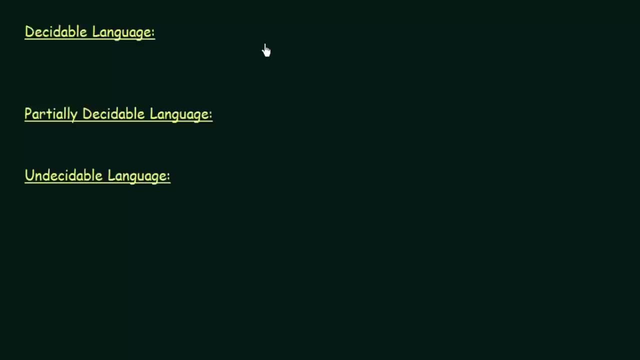 decidable languages and undecidable languages. So now, since we have understood recursive languages and recursively enumerable languages, we are in a position to define and understand these three terms, which are decidable languages, partially decidable languages and undecidable languages. 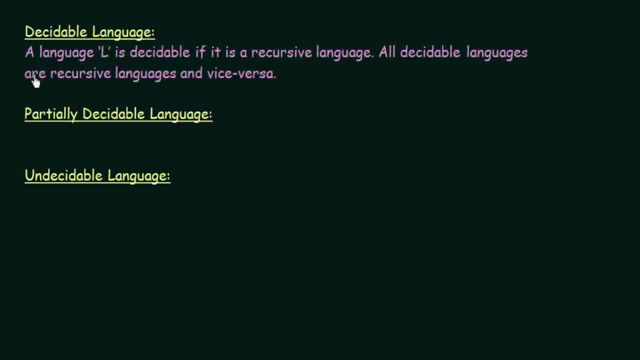 First let us see what are decidable languages. So it says a language L is decidable if it is a recursive language. All decidable languages are recursive languages and vice versa. Here it says that a language L is said to be decidable. 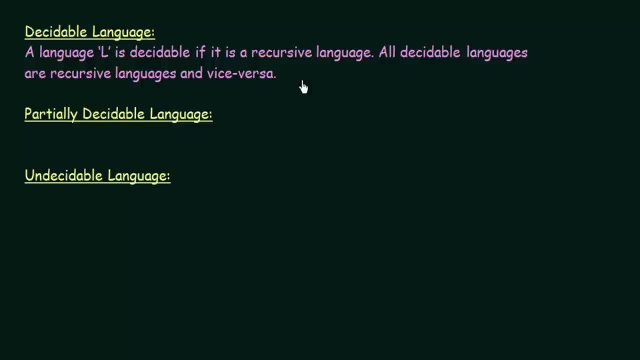 if it is a recursive language. We know what a recursive language is. Recursive languages are those in which the Turing machine will always hold. So if you have a language of which, if you pass any string to the Turing machine and the Turing machine always hold, 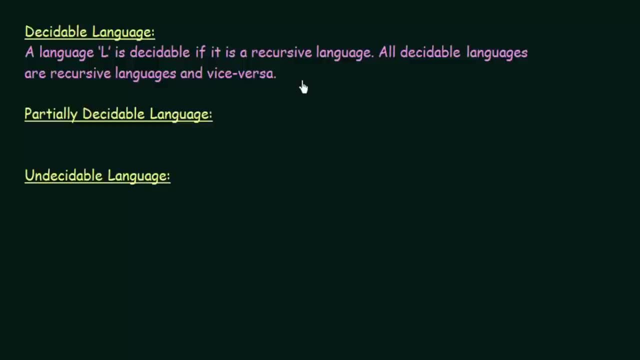 by either accepting or rejecting, then that language is said to be a decidable language. Alright, now let's see what is partially decidable language. So a language L is partially decidable if L is a recursively enumerable language. So we already know what is recursively enumerable language. 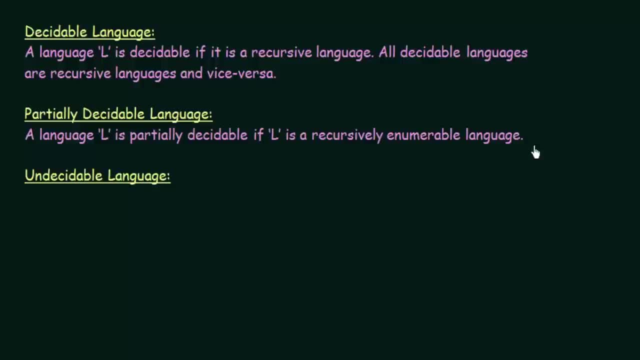 In recursively enumerable language, the Turing machine will sometimes hold and sometimes it will not hold. So those languages are known as partially decidable languages. So for both these two cases we see that there is a Turing machine for these two languages. 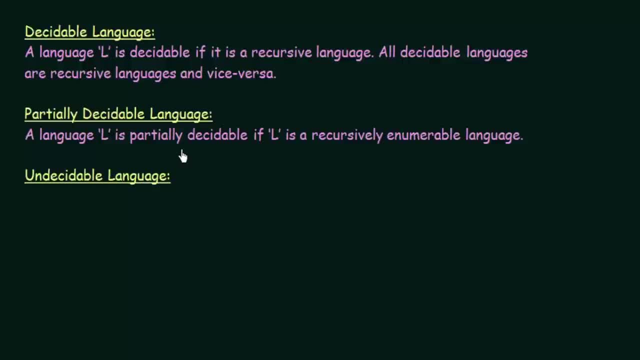 In one case, a Turing machine will always hold, and in the other case it will sometimes hold and sometimes not hold. So now I think you are getting an idea of what will be undecidable languages. So let's see what they are. 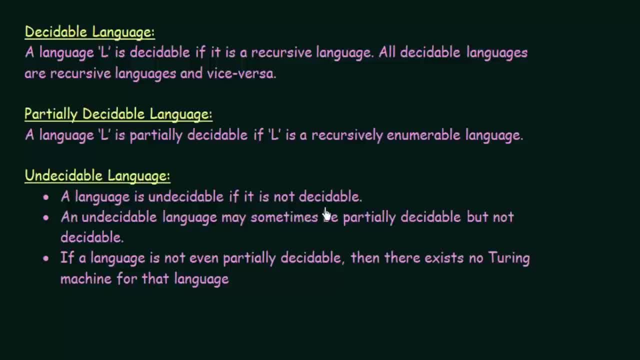 So a language is undecidable if it is not decidable. And what do we mean by this? An undecidable language may sometimes be partially decidable but not decidable. And if a language is not even partially decidable, then there exists no Turing machine for that language. 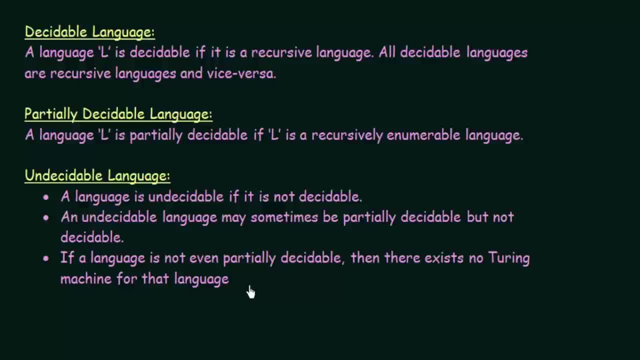 So we call a language undecidable when it is not decidable. And we know what is the meaning of decidable. We already studied here. So if it is not decidable, then it could be an undecidable language. 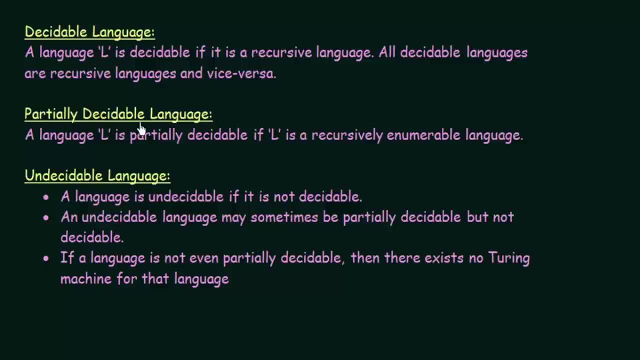 But there is a possibility that it can also be a partially decidable language. So when the Turing machine holds sometimes and does not hold in other times, in that time we call that it is a partially decidable language. But if a language is not even partially decidable, 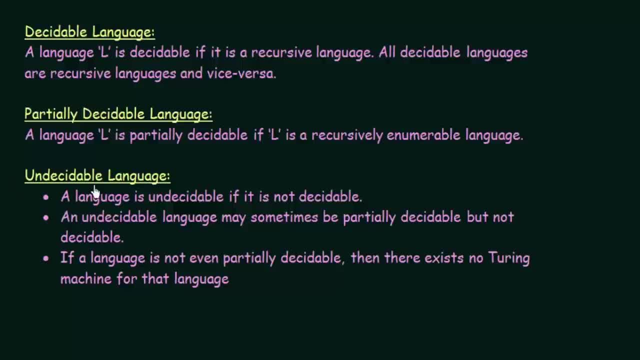 then that language is an undecidable language. If a language is not even partially decidable, then that is an undecidable language and there is no Turing machine for that language. We cannot design a Turing machine that will decide or that will recognize that language.